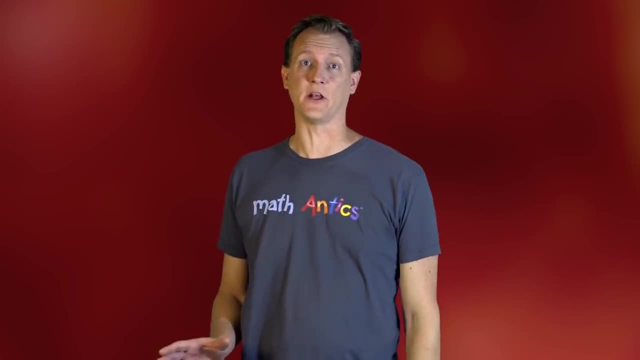 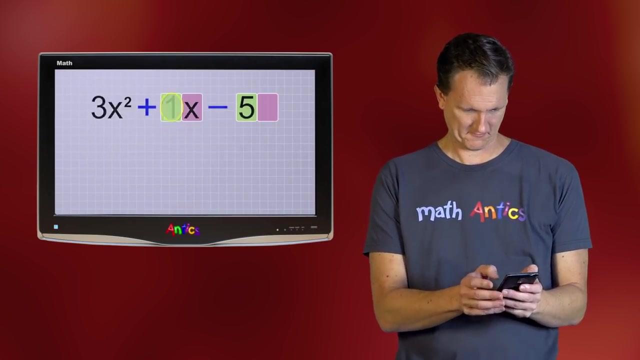 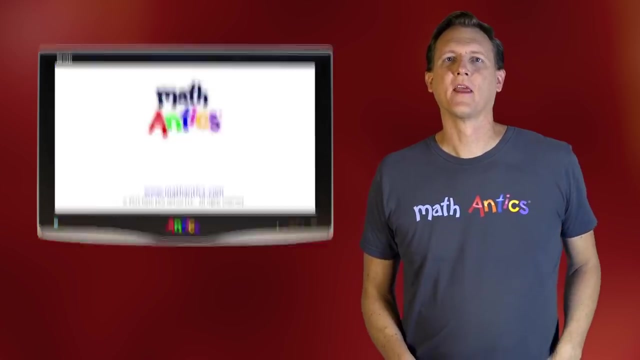 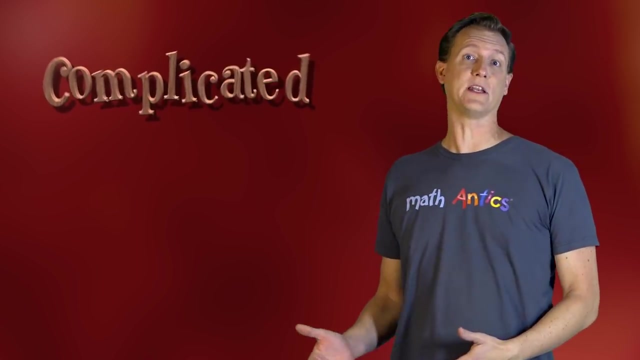 And if you don't remember much about polynomials, you might want to re-watch the first video before you continue. Go ahead, I'll wait. But even though the basics of polynomials are pretty simple, sometimes you'll come across polynomials that are more complicated than they really need to be. 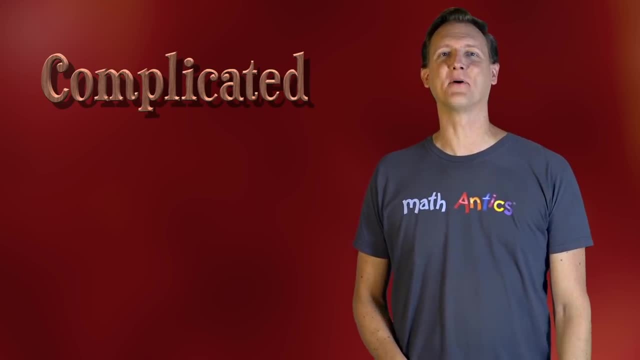 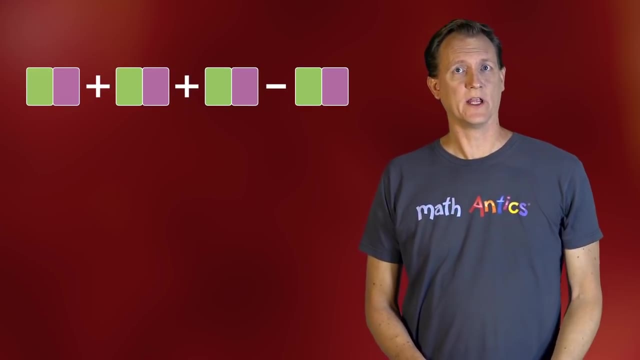 And in math, what do we like to do when things are too complicated? Yup, we simplify. So in this video, we're going to learn how to simplify polynomials. Simplifying a polynomial involves identifying terms that are similar enough that they can. 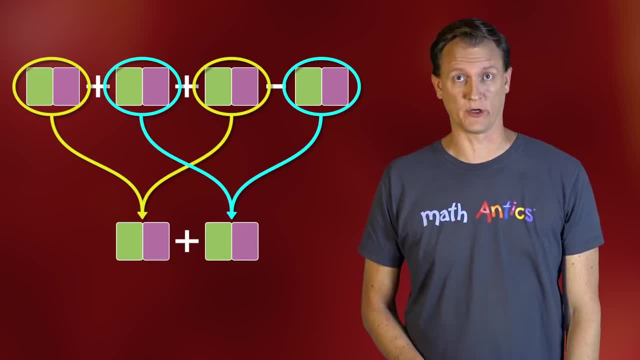 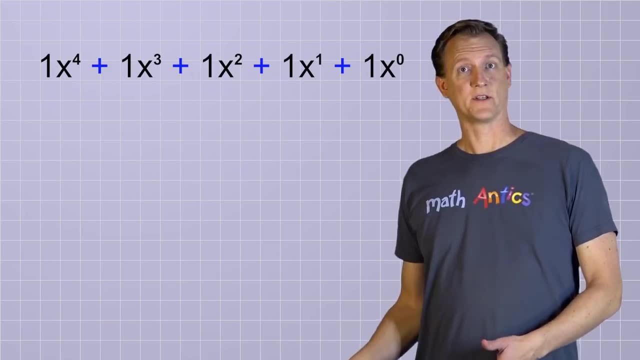 be combined into a single term to make the polynomial shorter. To see how that works, have a look at this basic polynomial that follows an easy-to-recognize pattern. Of course, as I mentioned in the last video, we don't really need to show the coefficients. 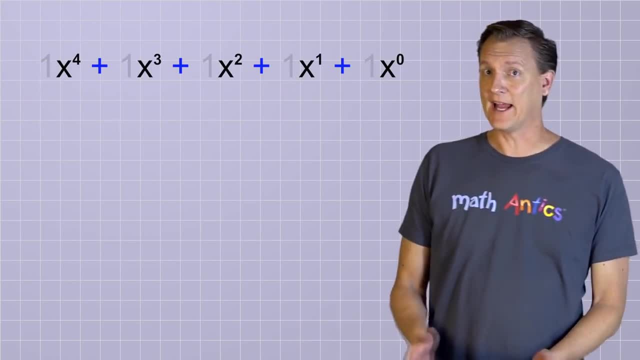 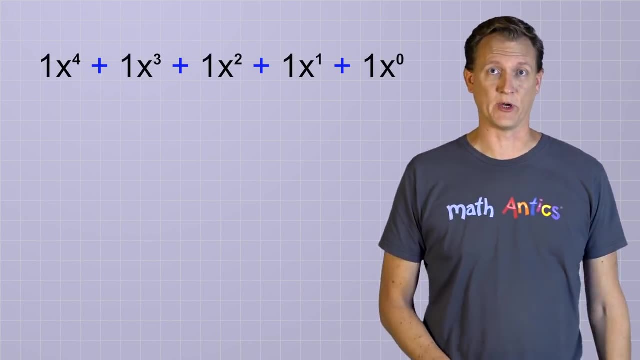 of each term if they're just one, like we have here, And the x to the zero term is also just one. So we don't really need to show that either, But I'm going to leave it like this just for a minute to illustrate my point. 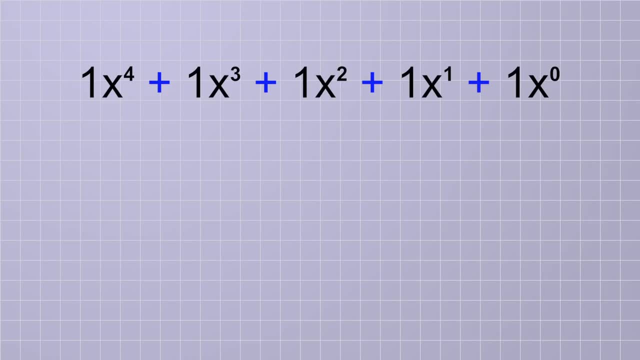 As you can see, this polynomial has a term of every degree, from zero up to four. But do you remember that it was okay for a polynomial to have missing terms? For example, we could have a slightly different polynomial that doesn't have a third degree term. 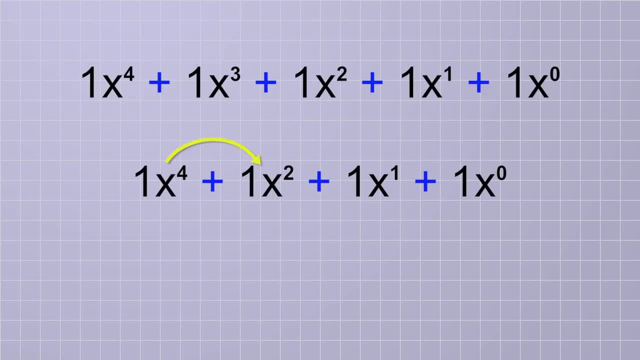 That makes it look like the x cubed term gets skipped or is missing, since the pattern goes from x to the fourth, then skips x cubed and goes to x squared, And so on. Well, just like there can be missing terms in a polynomial, there can also be extra terms. 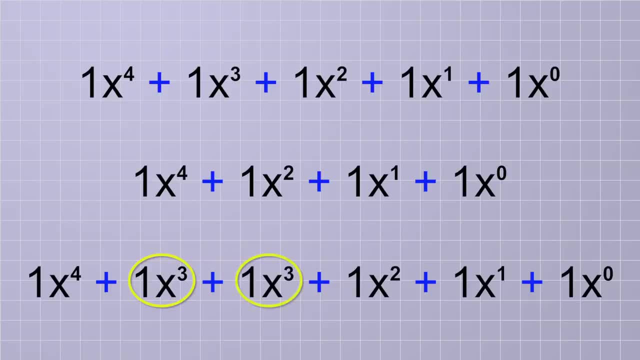 like in this polynomial, where the third degree term has been duplicated. See how there's two terms that have an x cubed variable part in this polynomial. So this polynomial has no x cubed term, which is fine, And this polynomial has just one x cubed term, which is fine. 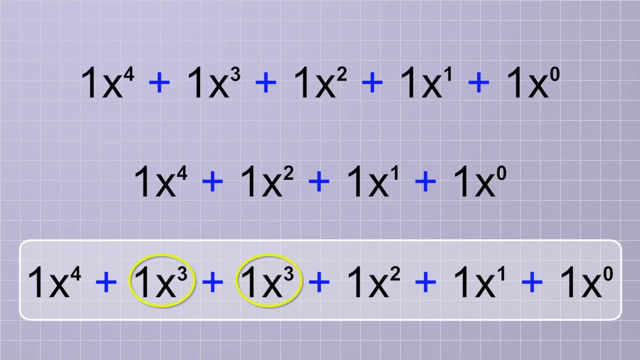 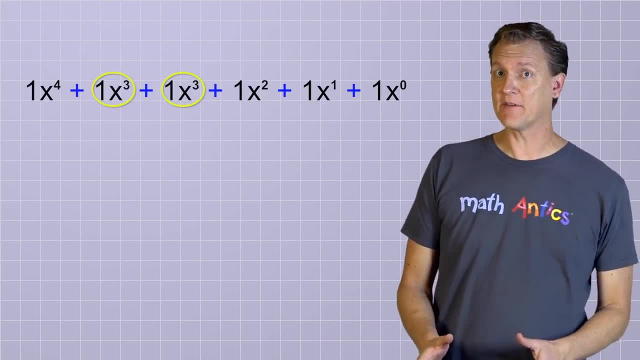 But this polynomial has two x cubed terms, which is also fine, But… It's more complicated than it needs to be, And whenever you have terms like this, terms that have the exact same variable part, they can be combined into a single term. 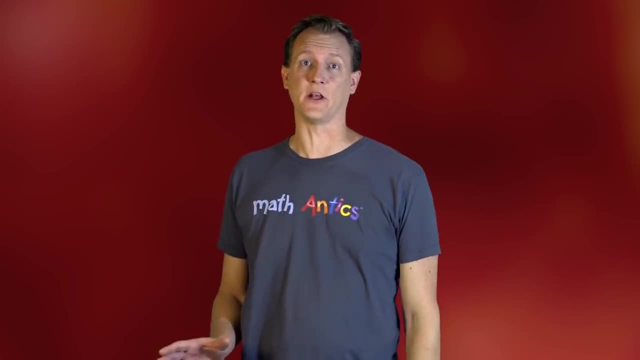 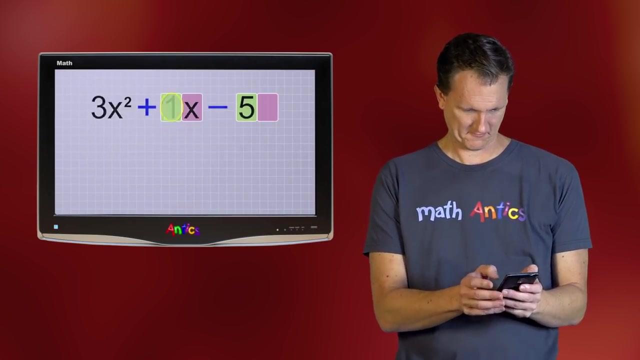 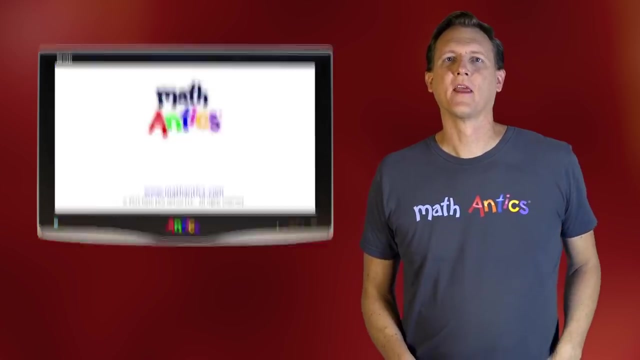 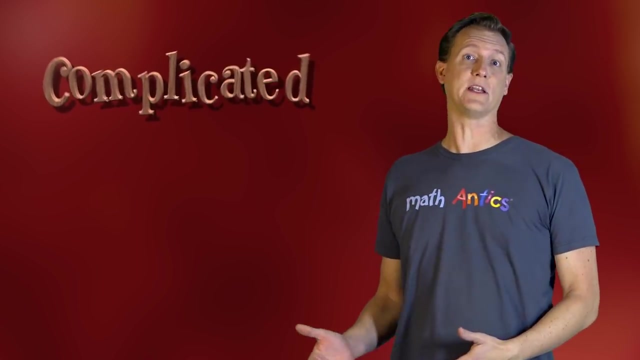 And if you don't remember much about polynomials, you might want to re-watch the first video before you continue. Go ahead, I'll wait. But even though the basics of polynomials are pretty simple, sometimes you'll come across polynomials that are more complicated than they really need to be. 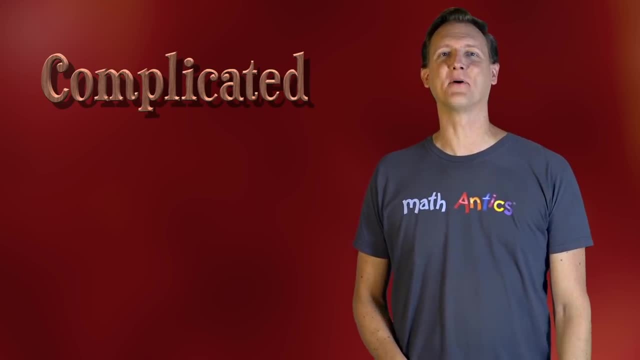 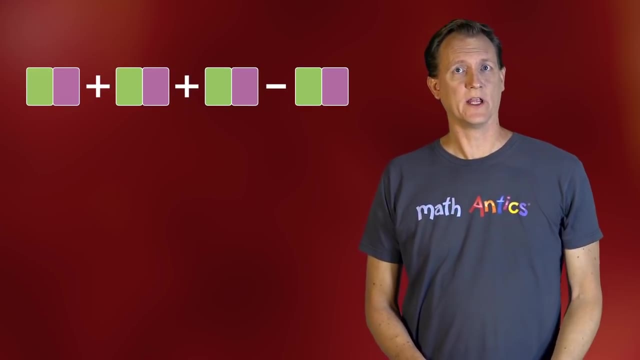 And in math, what do we like to do when things are too complicated? Yup, we simplify. So in this video, we're going to learn how to simplify polynomials. Simplifying a polynomial involves identifying terms that are similar enough that they can. 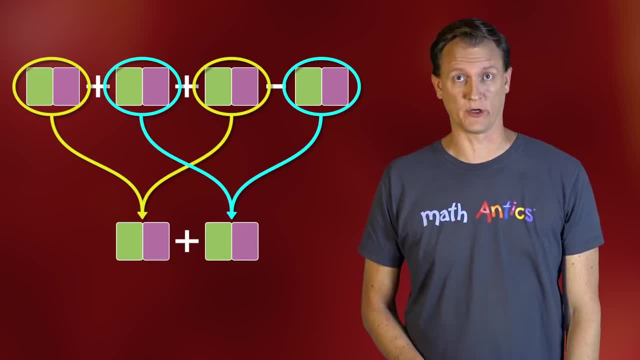 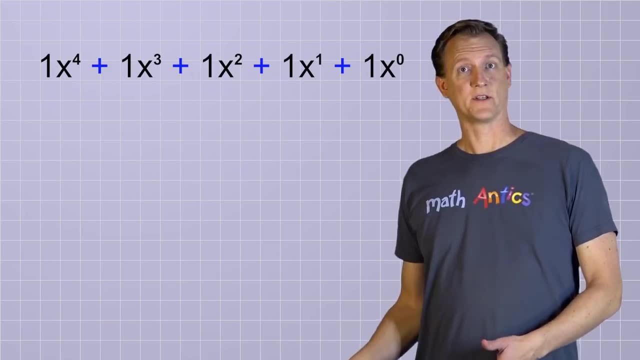 be combined into a single term to make the polynomial shorter. To see how that works, have a look at this basic polynomial that follows an easy-to-recognize pattern. Of course, as I mentioned in the last video, we don't really need to show the coefficients. 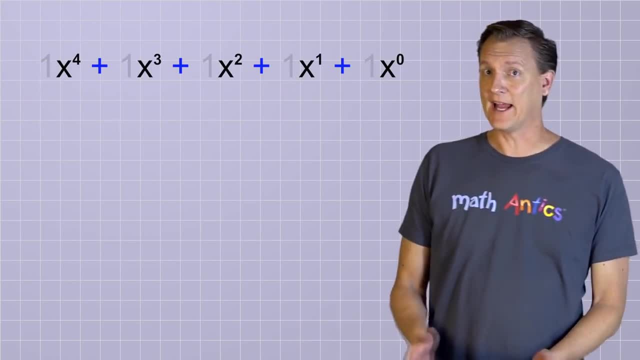 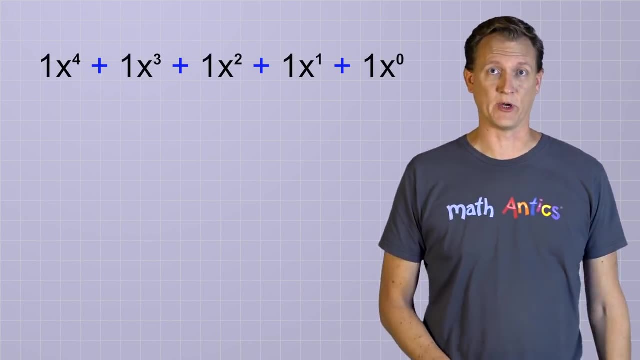 of each term if they're just one, like we have here, And the x to the zero term is also just one. So we don't really need to show that either, But I'm going to leave it like this just for a minute to illustrate my point. 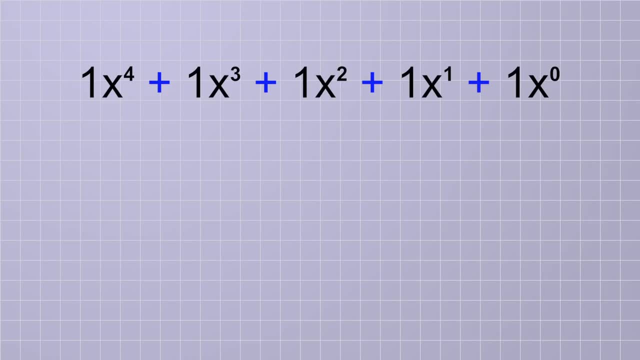 As you can see, this polynomial has a term of every degree, from zero up to four. But do you remember that it was okay for a polynomial to have missing terms? For example, we could have a slightly different polynomial that doesn't have a third-degree term. 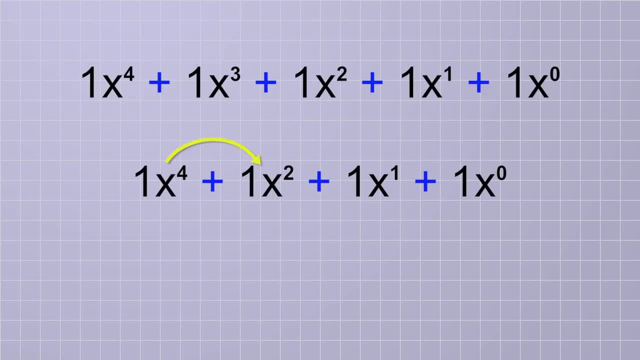 That makes it look like the x cubed term gets skipped or is missing, since the pattern goes from x to the fourth, then skips x cubed and goes to x squared, And so on. Well, just like there can be missing terms in a polynomial, there can also be extra terms. 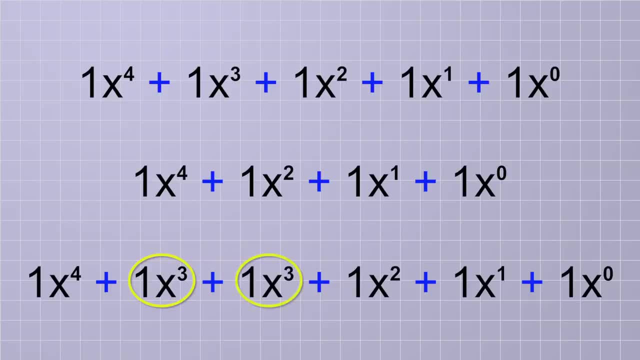 like in this polynomial where the third-degree term has been duplicated. See how there's two terms that have an x cubed variable part in this polynomial. So this polynomial has no x cubed term, which is fine, And this polynomial has just one x cubed term, which is fine. 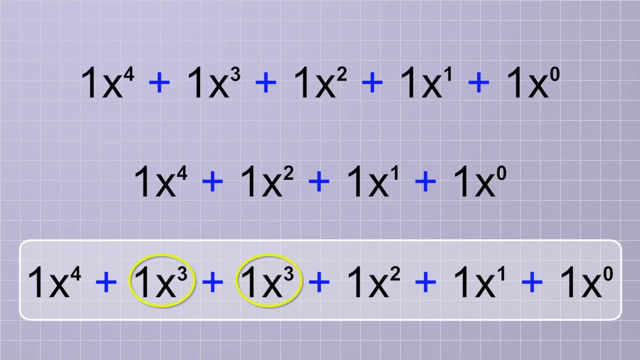 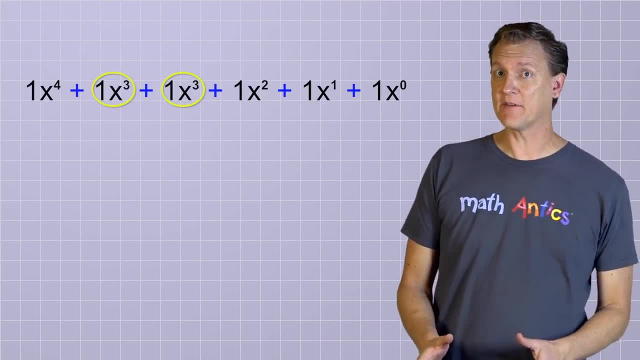 But this polynomial has two x cubed terms, which is also fine, But… It's more complicated than it needs to be, And whenever you have terms like this, terms that have the exact same variable part, they can be combined into a single term. 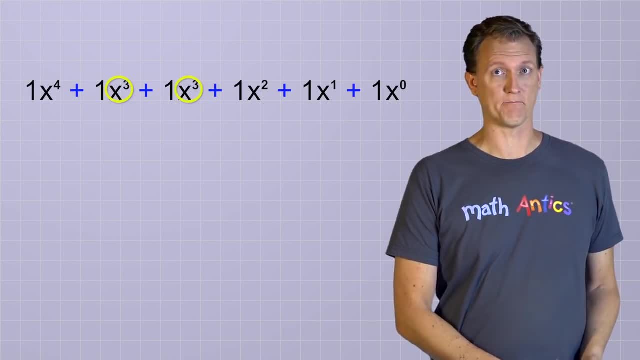 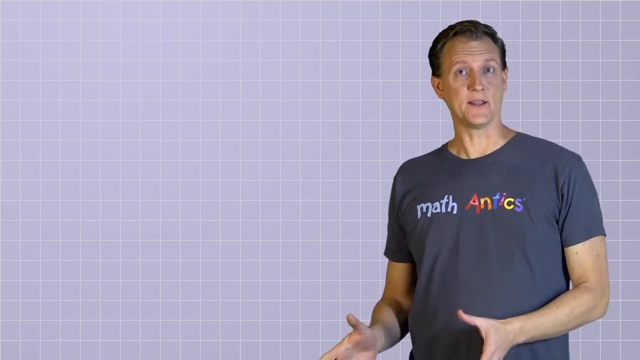 To do that you just add the number parts and you keep the variable part the same. So 1x cubed plus 1x cubed combine to form 2x cubed. What we just did there is called combining like terms. 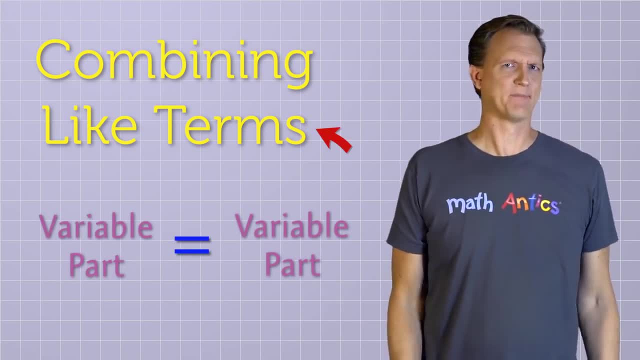 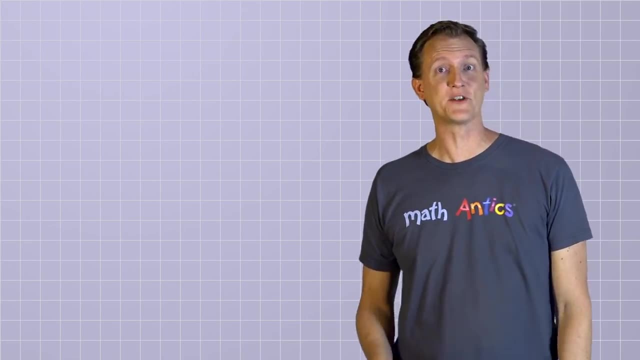 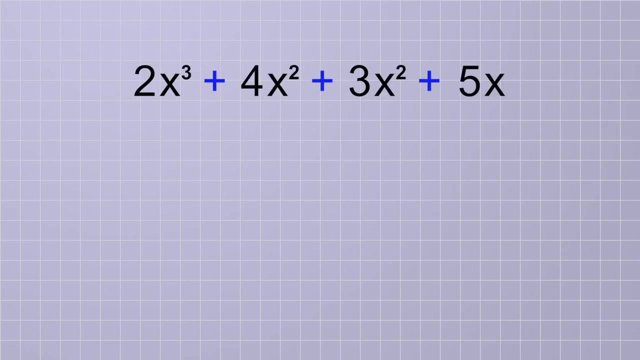 Like terms are terms that have exactly the same variable part. But why can we combine them? Well, to understand that… I like to pretend that the variable parts of a polynomial's terms are fruit. Yes, you heard me… fruit, For example. have a look at this polynomial. 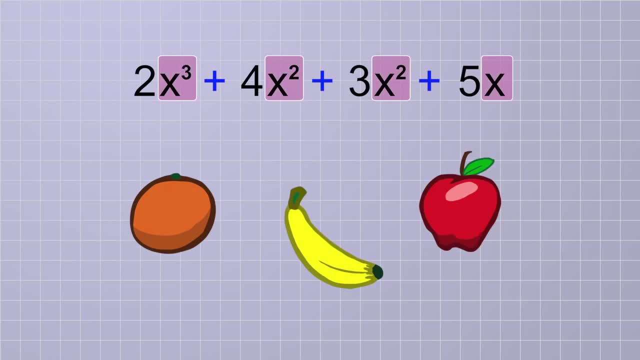 But let's substitute a different kind of fruit for each different variable part. Let's change x cubed to apples, x squared to oranges and just plain x to bananas. If we do that, what would this new fruit polynomial be telling us? 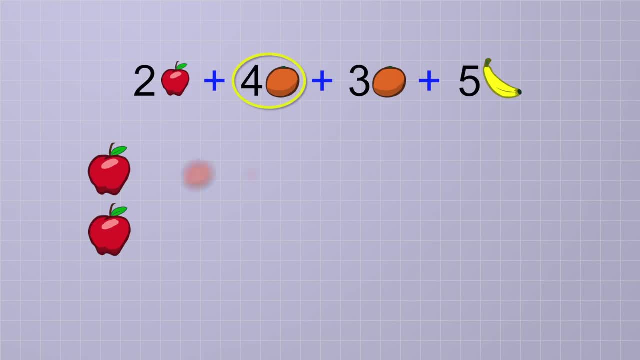 Well, this first term represents two apples, The next term is four oranges, The next term is three oranges And the last term is five bananas, And these are all being added together. So that raises the question: what do you get when you add two apples to four oranges? 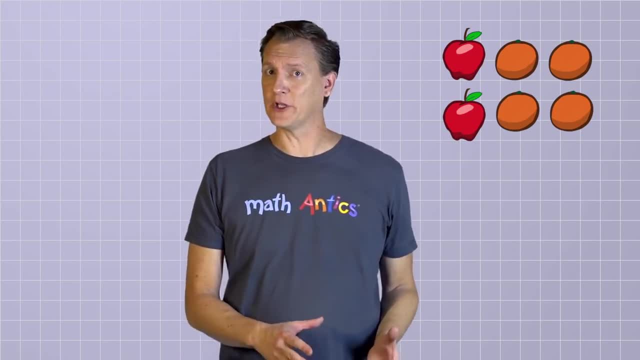 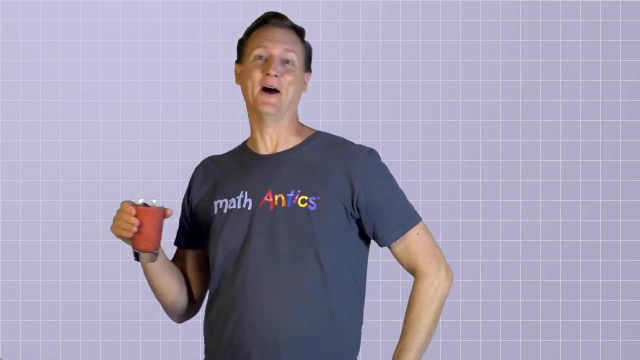 Well, you get two apples and four oranges. Since they're different fruit, you can't combine them Well, unless you have a blender. that is Ah, but what about the middle two terms? What do we get if we add four oranges to four oranges? 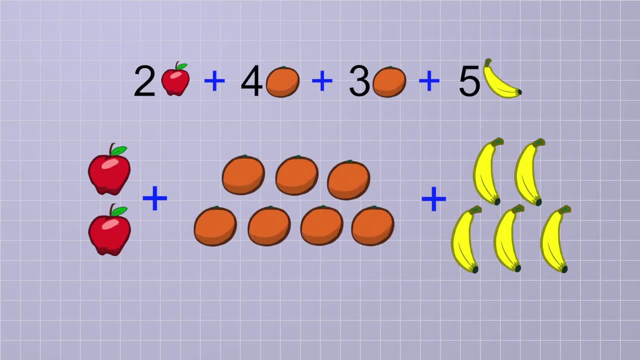 Well, what about the middle two terms? Well, we get three oranges and three oranges. That's easy… seven oranges. And that means we CAN combine these two terms into a single term, which makes our fruit polynomial simpler. Now do you see why the variable parts of a term have to be exactly the same in order? 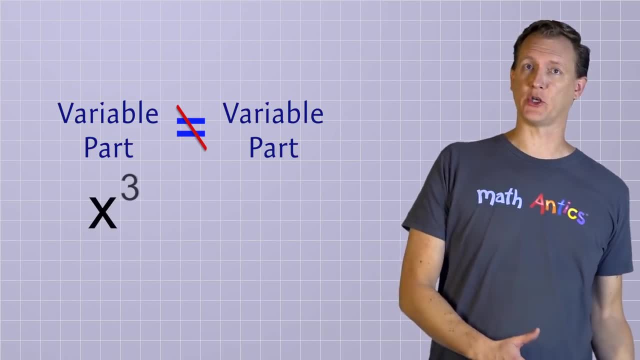 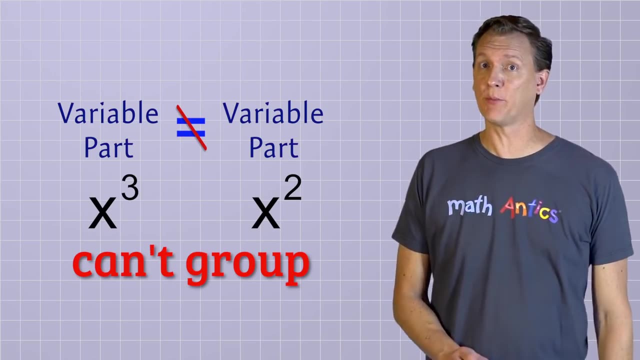 to combine them. If the variable parts are different, like x cubed and x squared, then they represent different things. so we can't group them into a single term the way that we can if the variable parts are the same. The mathematical reason that it works that way has to do with something called…. 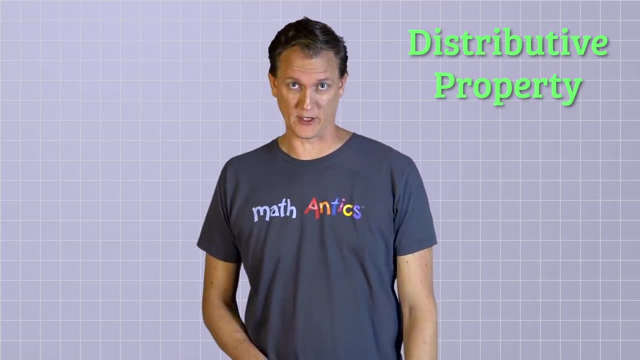 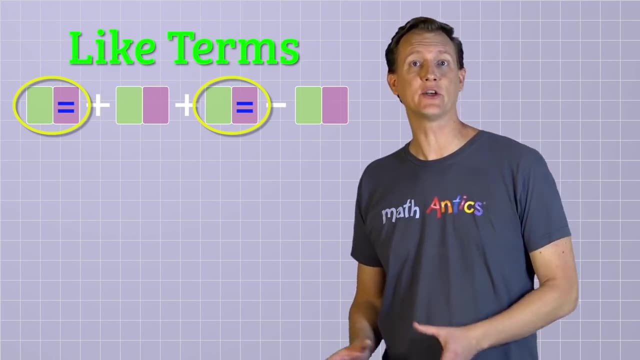 called the Distributive Property, which is the subject of a whole other video. Alright, so if two terms in a polynomial have exactly the same variable part, then we call them like terms and we can combine them into a single term to simplify the polynomial. 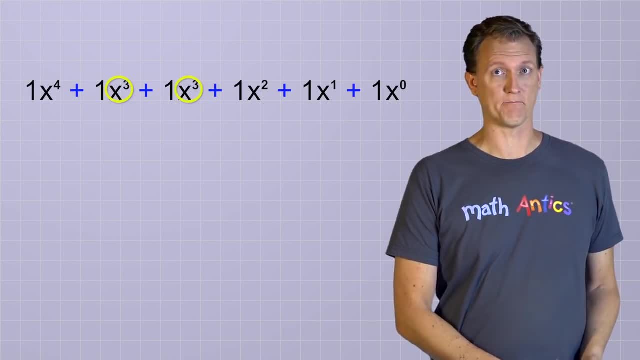 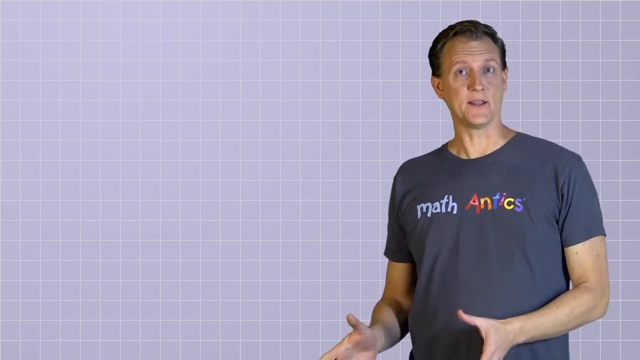 To do that you just add the number parts and you keep the variable part the same. So 1x cubed plus 1x cubed combine to form 2x cubed. What we just did there is called combining like terms. 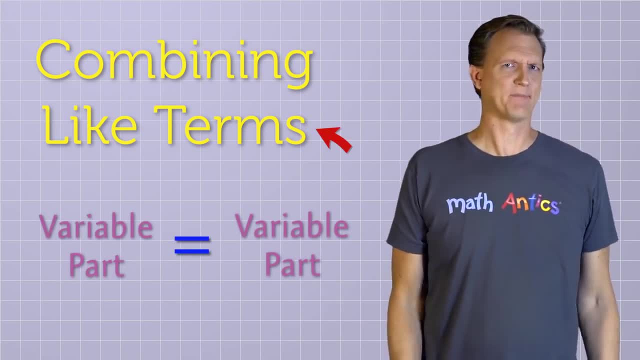 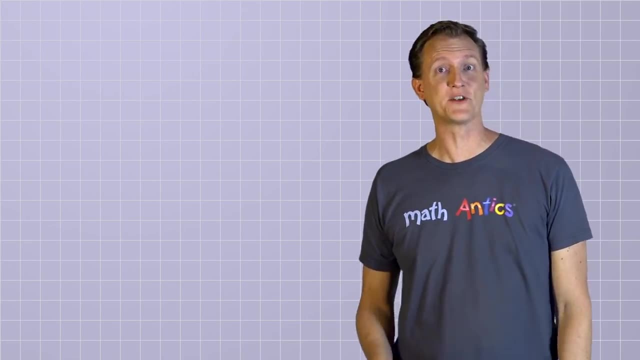 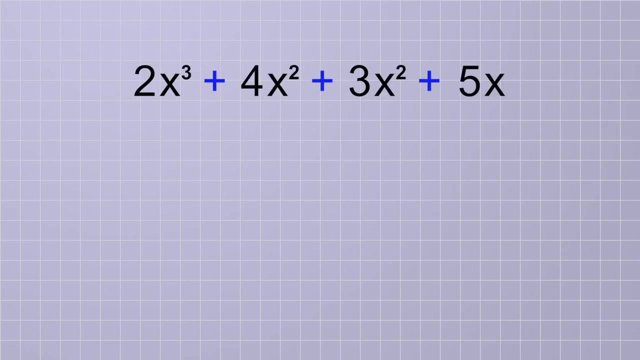 Like terms are terms that have exactly the same variable part. But why can we combine them? Well, to understand that… I like to pretend that the variable parts of a polynomial's terms are fruit. Yes, you heard me… fruit, For example. have a look at this polynomial. 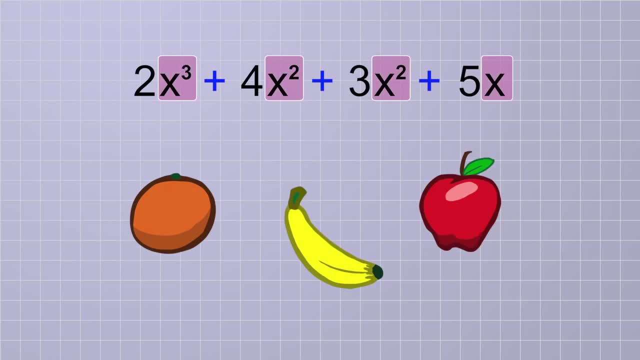 But let's substitute a different kind of fruit for each different variable part. Let's change x cubed to apples, x squared to oranges and just plain x to bananas. If we do that, what would this new fruit polynomial be telling us? 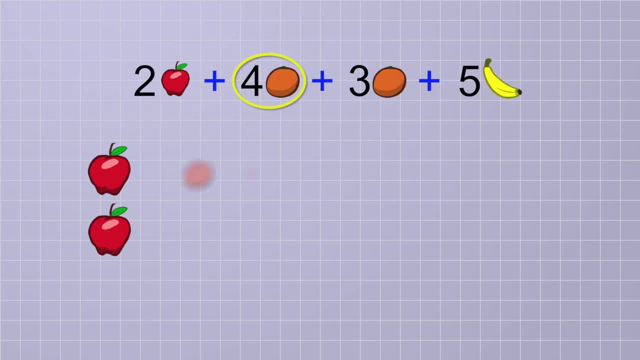 Well, this first term represents two apples, The next term is four oranges, And this first term represents two apples, The next term is three oranges And the last term is five bananas, And these are all being added together. So that raises the question…. 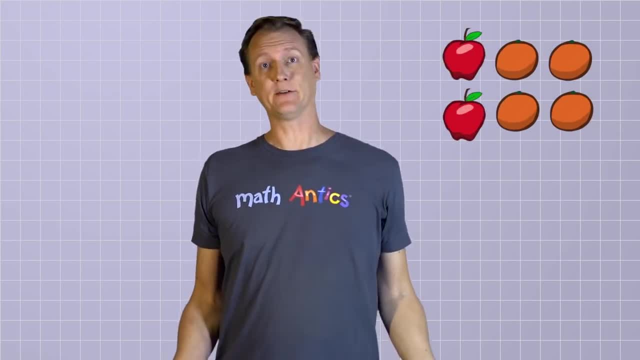 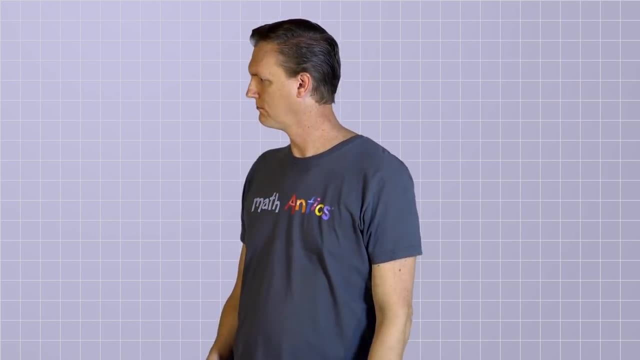 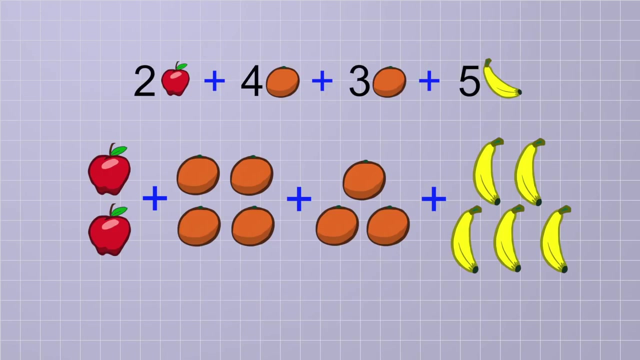 What do you get when you add two apples to four oranges? Well, you get two apples and four oranges. Since they're different fruit, you can't combine them. Well, unless you have a blender. that is, Ah, but what about the middle two terms? 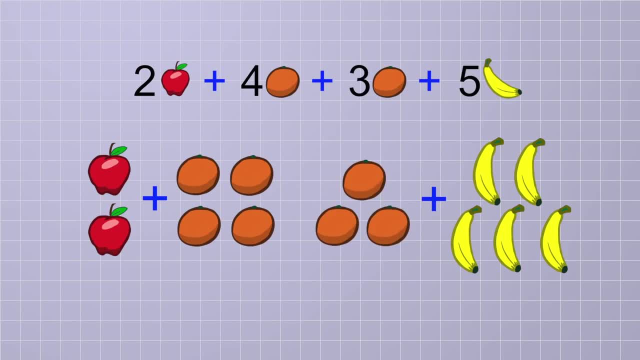 What do we get if we add four oranges to four oranges? We get four oranges and three oranges. That's easy… seven oranges. And that means that we CAN combine these two terms into a single term, which makes our fruit polynomial simpler. Now do you see why the variable parts of a term have to be EXACTLY the same in order? 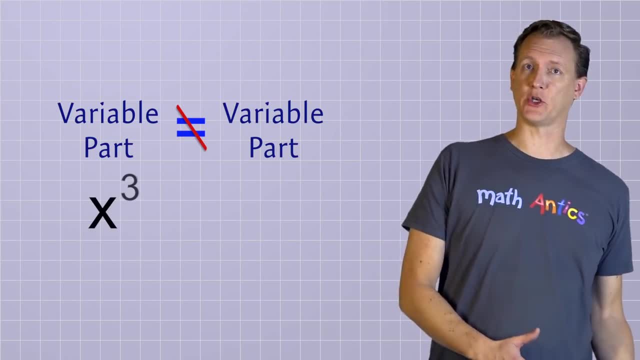 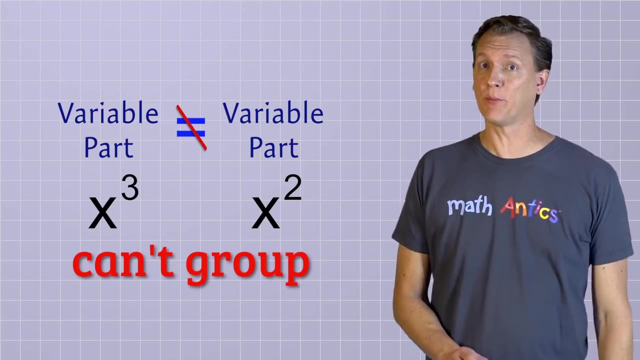 to combine them. If the variable parts are different, like x cubed and x squared, then they represent different things. So we can't group them into a single term the way that we can if the variable parts are the same. The mathematical reason that it works that way has to do with something that we don't. 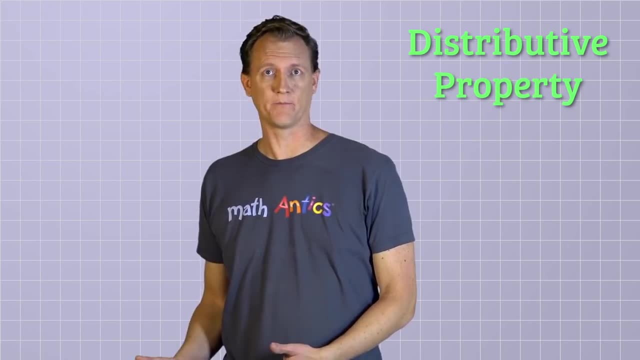 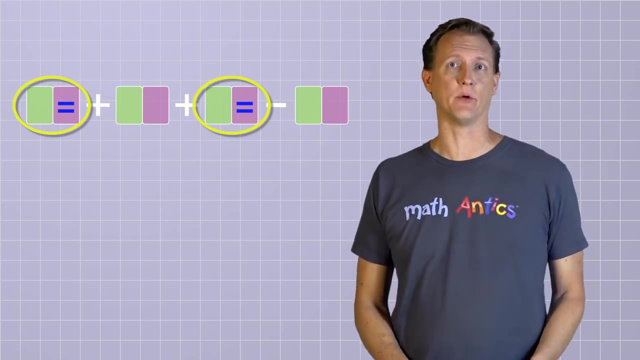 know yet. So let's look at this. It has to do with something called the Distributive Property, which is the subject of a whole other video. Alright, so if two terms in a polynomial have exactly the same variable part, then we call. 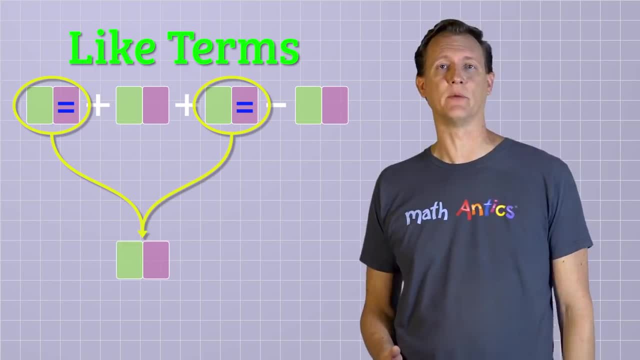 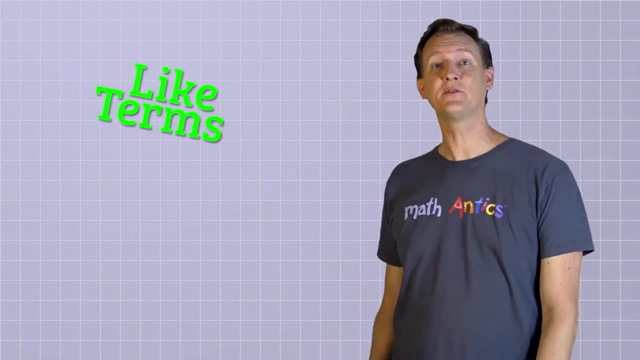 them like terms and we can combine them into a single term. to simplify the polynomial And to help you get better at identifying like terms, let's play a little game called Like Terms or Not Like Terms. The first pair of terms we'll consider is 2x and 3x. 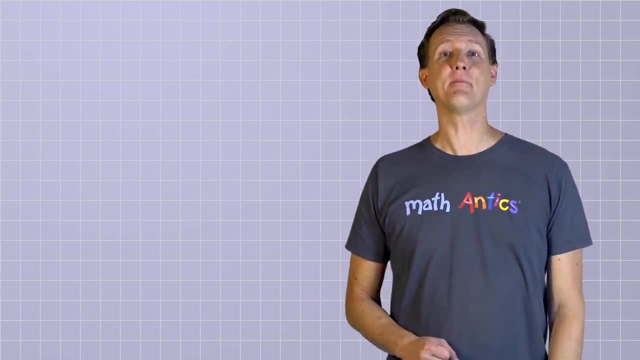 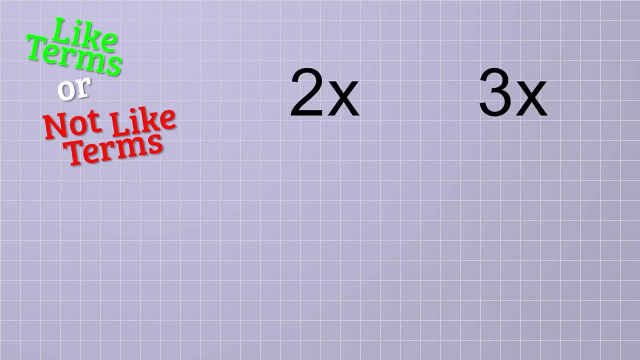 And to help you get better at identifying like terms, let's play a little game called Like Terms or Not Like Terms. The first pair of terms we'll consider is 2x and 3x. Are they like terms? Yep, The variable part of both terms is the same x, so we can combine them into a single term. 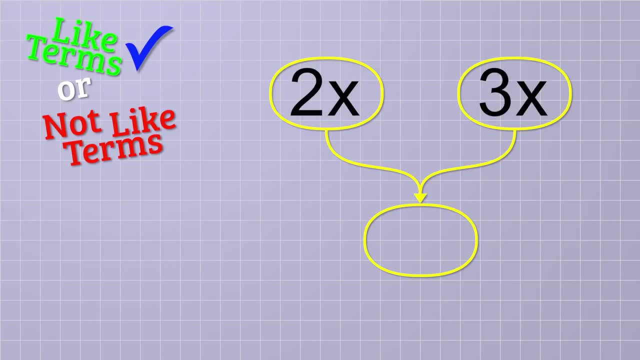 We do that by adding the number parts and keeping the variable part the same. 2 plus 3 is 5, so the combined term is 5x. Next up we have 4x and 5y. Are these like terms? 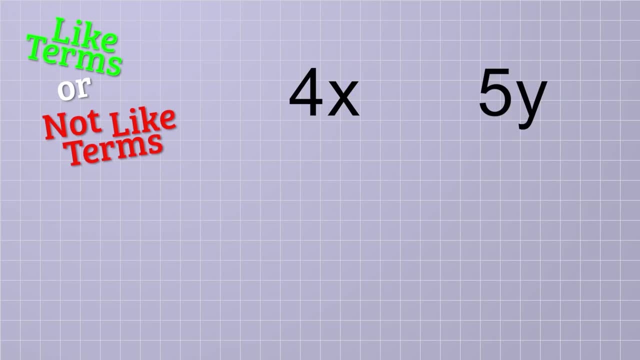 Well, they're both first degree terms, but since the variables are different letters, they are NOT like terms. That means we can't combine them. OK, but what about these terms 2x squared and negative 7x squared? Well, the variable part in both is exactly the same: it's x squared. 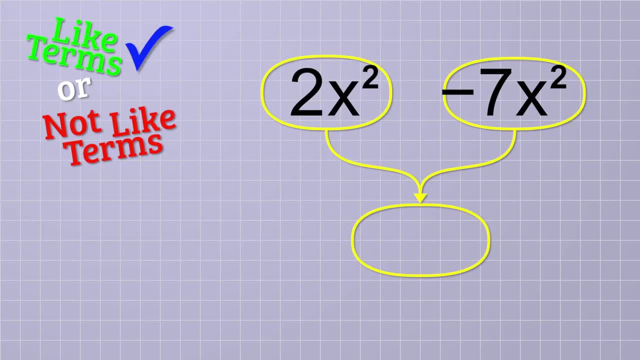 So, yes, these are like terms and we can combine them. Notice that one of the terms is negative, so when we add the number parts, we'll end up with negative 5. So these combine to negative 5x squared. Our next pair of terms is 4x squared and 6x cubed. 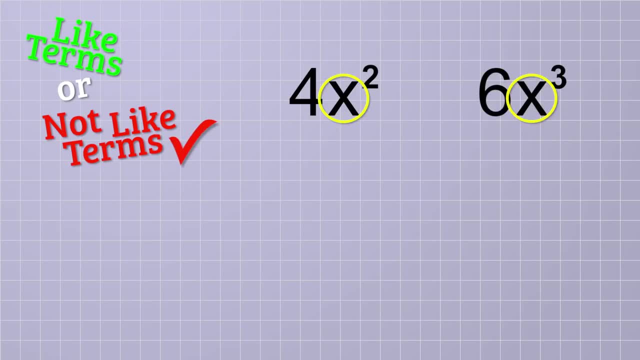 Are these like terms? Nope, Even though the variable is x, in both cases the exponents are 2x squared and 6x squared. Are these like terms? Nope, The exponents are different, so the variable parts are NOT the same. 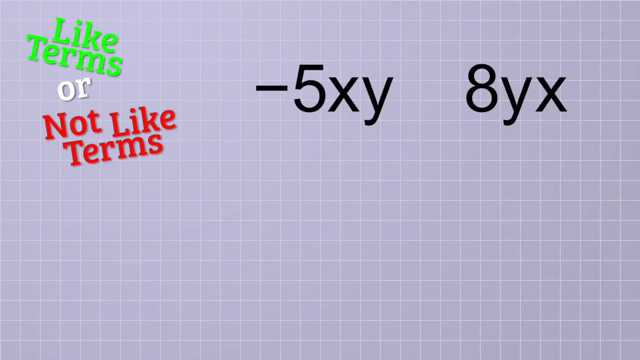 Next we have negative 5xy and 8yx. Are these like terms? Well, at first glance you might think that the variable parts of these terms are different because the x and the y are in a different order. But remember, multiplication has the commutative property, so the order doesn't matter. 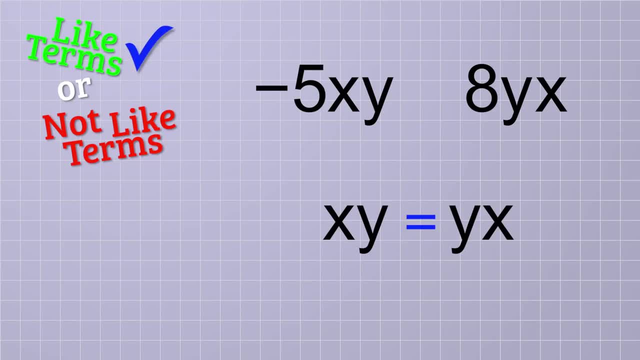 xy is the same as yx, so we can rewrite them so that they look the same too. There Add the number parts Negative. 5 plus 8 is 3.. So we wind up with the single term, 3xy. Last we have 5x squared y and 5y squared x. 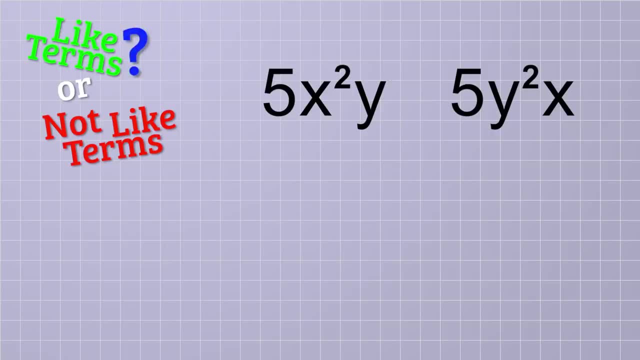 Now be careful with this one. You might think that it's like the last one, where the terms are just in a different order, But look closely. In the first term the x is being squared, but in the second term the y is being squared. 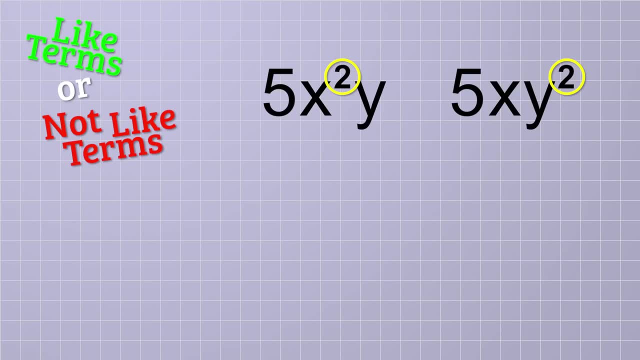 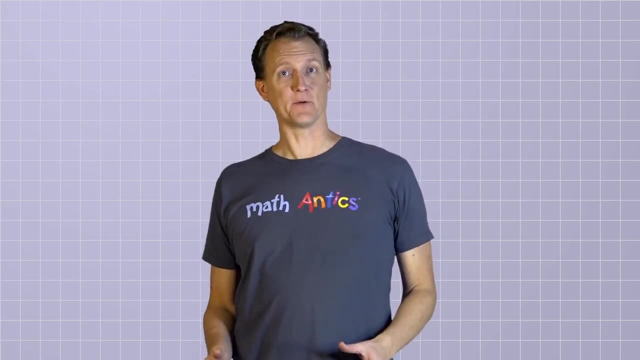 That means even if we switch the order, the exponents move with the variables, so the variable parts are not the same, Which means these are NOT like terms. Alright, now that you've had some practice identifying like terms, let's look at some. 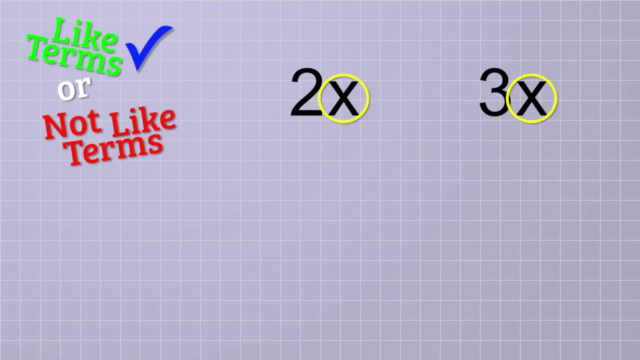 Are they like terms? Yep, The variable part of both terms is the same x, so we can combine them into a single term. We do that by adding the number parts and keeping the variable part the same. 2 plus 3 is 5, so the combined term is 5x. 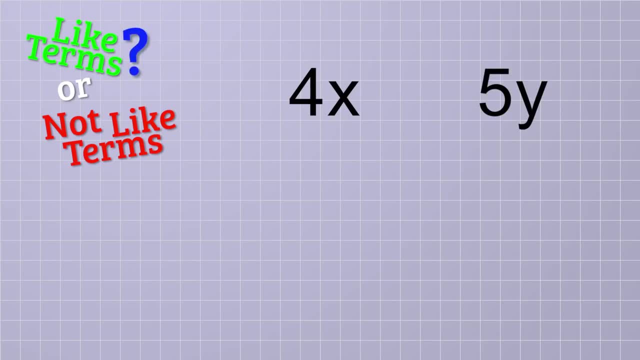 Next up we have 4x and 5y. Are these like terms? Well, they're both first degree terms, but since the variables are different letters, they are NOT like terms. That means we can't combine them. OK, but what about these terms? 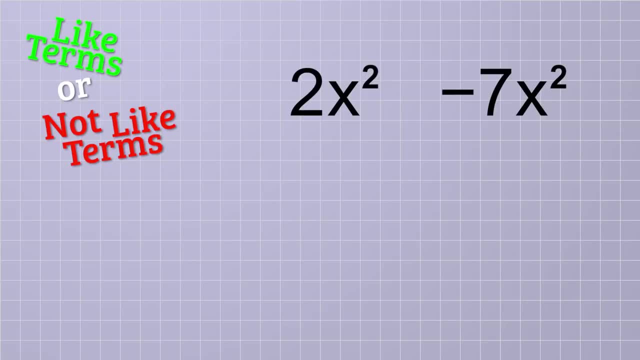 2x squared and negative. 3x Negative, 7x squared. Well, the variable part in both is exactly the same: it's x squared. So, yes, these are like terms and we can combine them. Notice that one of the terms is negative. so when we add the number parts, we'll end. 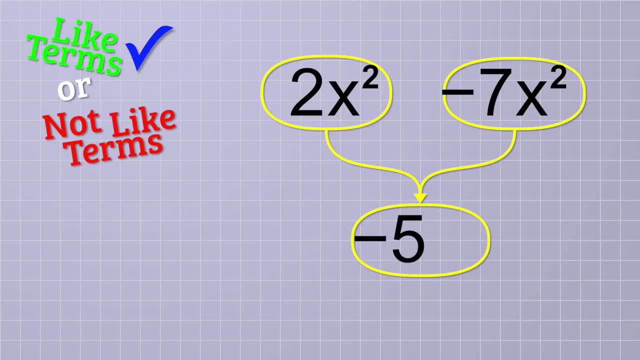 up with negative 5.. So these combine to negative: 5x squared. Our next pair of terms is 4x squared and 6x cubed. Are these like terms? Nope, Even though the variable is x, in both cases the exponents are different. 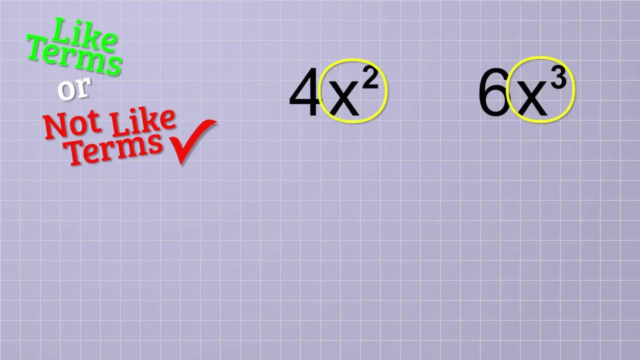 So the variable parts are NOT the same. Next we have negative 5xy and 8yx. Are these like terms? Well, at first glance you might think that the variable parts of these terms are different because the x and the y are in a different order. 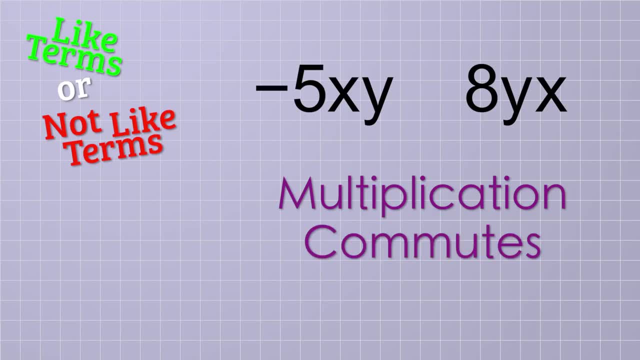 But remember, multiplication has the commutative property, so the order doesn't matter. xy is the same as yx, so we can rewrite them so that they look the same too. Now we can add the number parts Negative. 5 plus 8 is 3.. 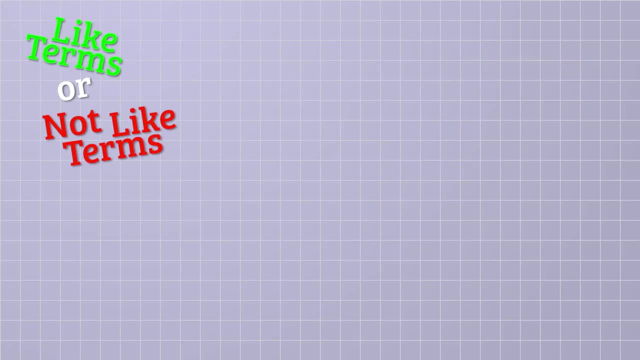 So we wind up with the single term 3xy. Last we have 5x squared y and 5y squared x. Now be careful with this one. You might think that it's like the last one, where the terms are just in a different. 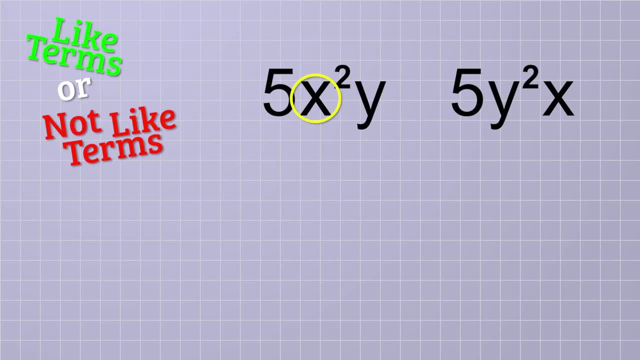 order. But look closely: In the first term the x is being squared, but in the second term the y is being squared. That means even if we switch the order, the exponents move with the variables, so the variable parts are not the same. 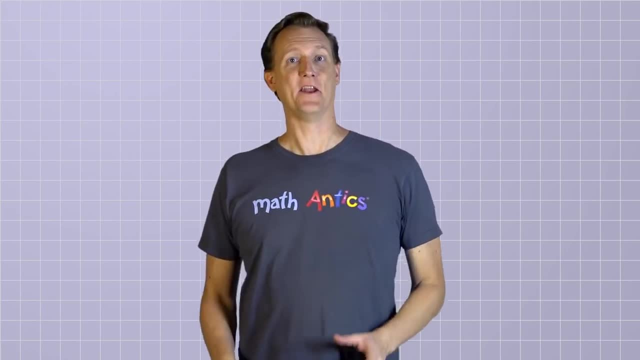 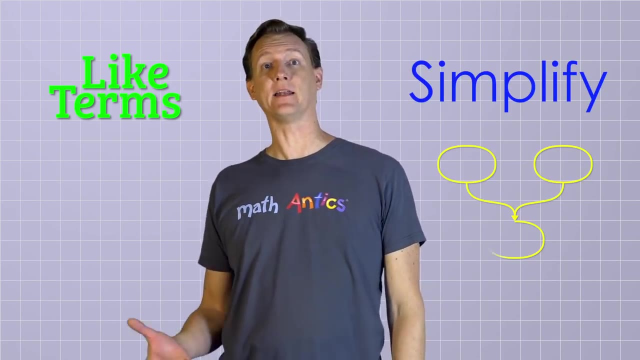 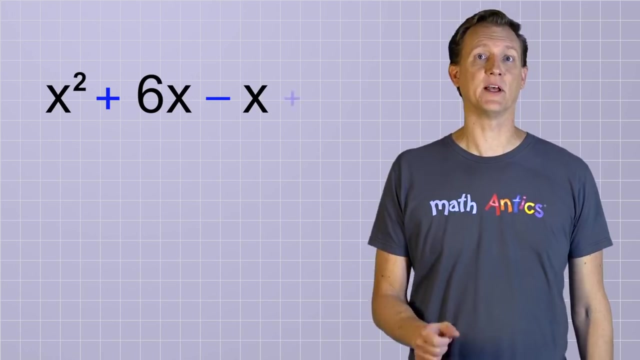 Which means these are NOT like terms. Alright, now that you've had some practice identifying like terms, let's look at some complicated polynomials that we can simplify by combining any like terms that we find. Here's our first example: x squared plus 6x minus x plus 10.. 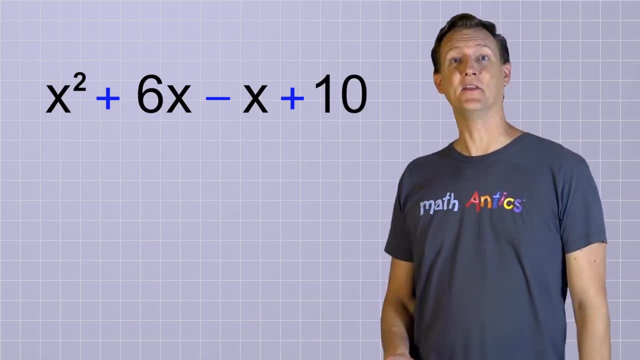 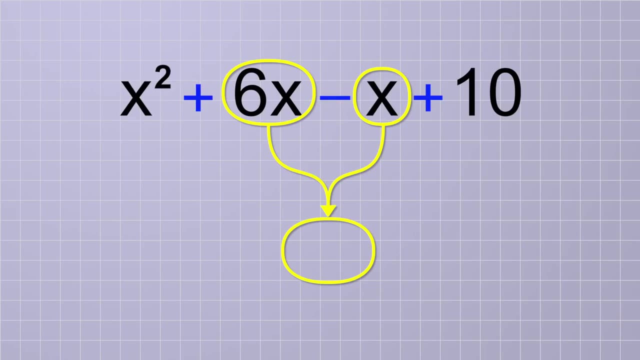 Do you see any terms that have the same variable part? Yup, these two terms in the middle both have the variable x, so we can combine them. 6x minus x would just give us 5x, since 6 minus 1 is 5.. 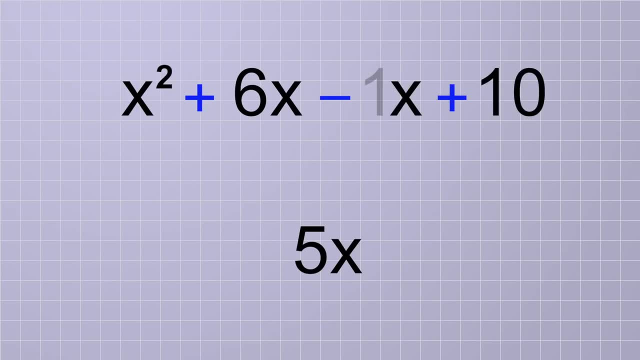 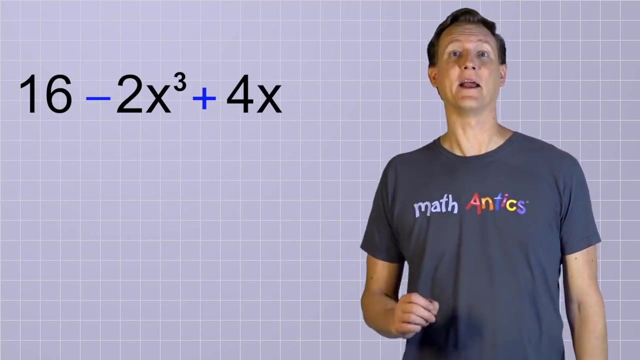 Remember, if you don't see a number part in a term, then it's just 1.. So this polynomial started with 4 terms, but simplified to 3 terms: x squared plus 5x plus 10.. Let's try this one: 16 minus 2x cubed plus 4x minus 10.. 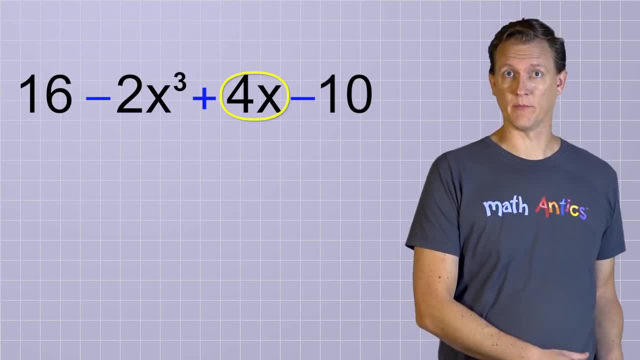 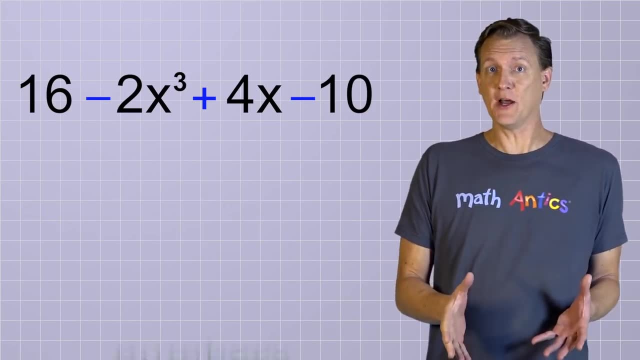 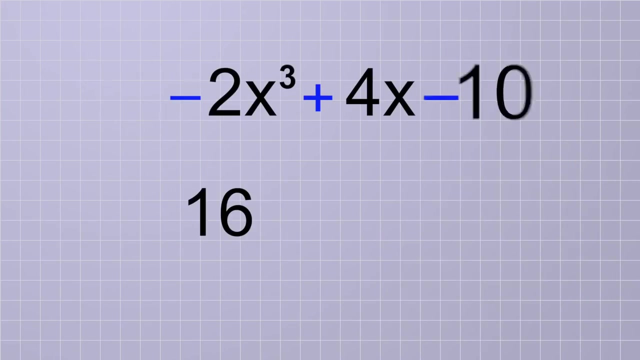 In this polynomial we have a third degree term, a first degree term and two constant terms. Are those constant terms like terms? Absolutely, They're both just numbers and don't really have a variable part. so we can combine them easily. This term is positive 16 and this term is negative 10, so if you add them together, you 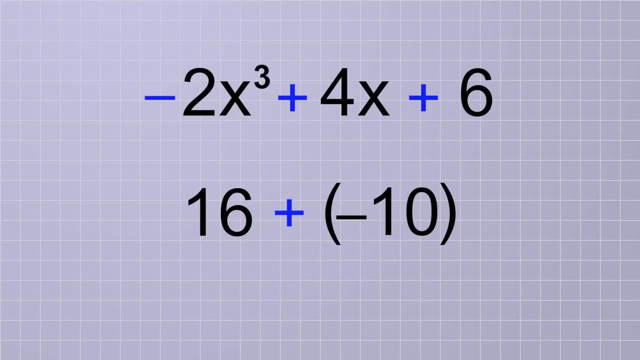 end up with positive 6.. Remember, it's best to think of all terms in a polynomial as being added, but they can have coefficients that are either positive or negative. That's why this negative sign stays here with the 2x cubed term, because it's a negative term. 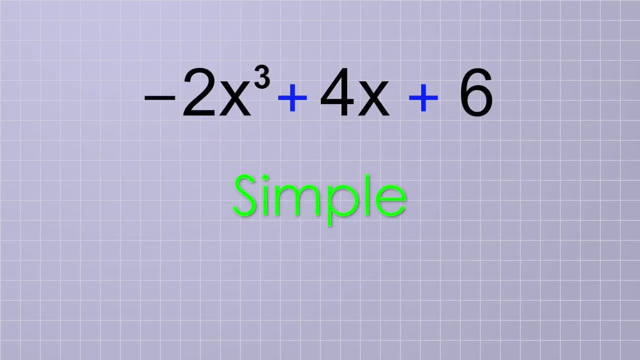 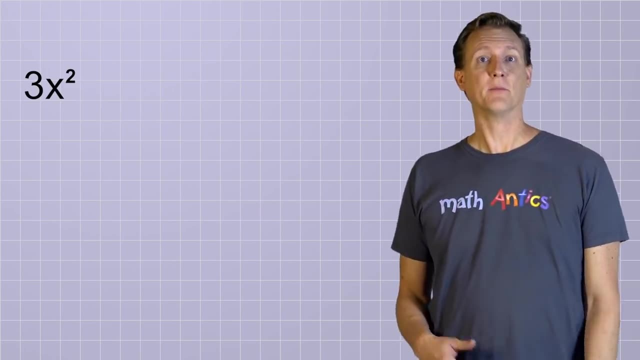 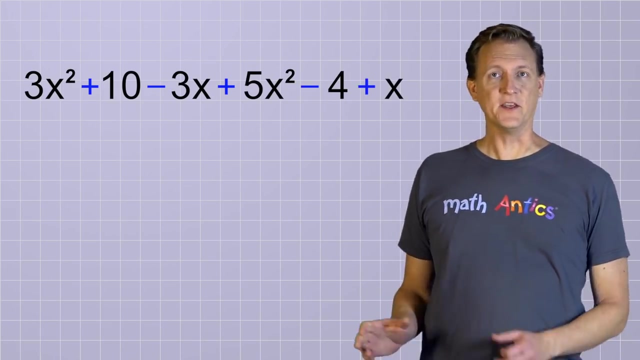 So this polynomial is now as simple as it can be, since there's no other like terms Ready for an even more complicated polynomial: 3x squared plus 10 minus 3x plus 5x squared minus 4 plus x. This polynomial has 6 terms, and when you get a long polynomial like this, the first: 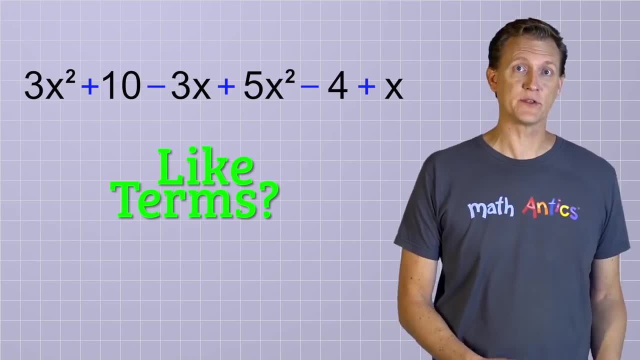 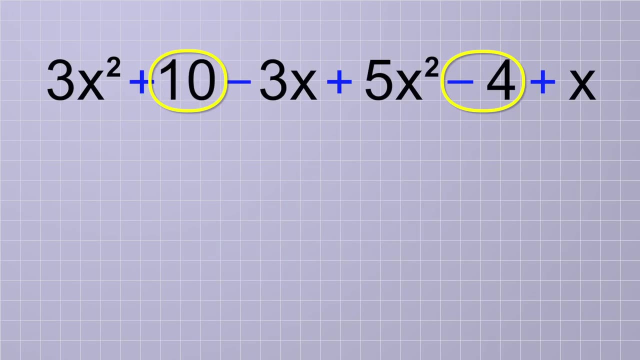 thing to do is look to see if any of the terms are like terms so you can combine them. Well… right away, you may notice…. …that there's two constant terms in this polynomial: positive 10 and negative 4.. So let's start by combining them into a single constant term: positive 6, since 10. 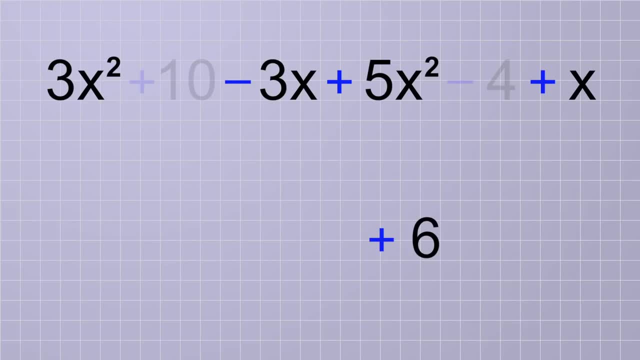 minus 4 equals 6.. Next we see that there are also two first degree terms, negative 3x and positive x. Those are like terms, so we can combine them. Negative 3x plus 1x gives us negative 2x. 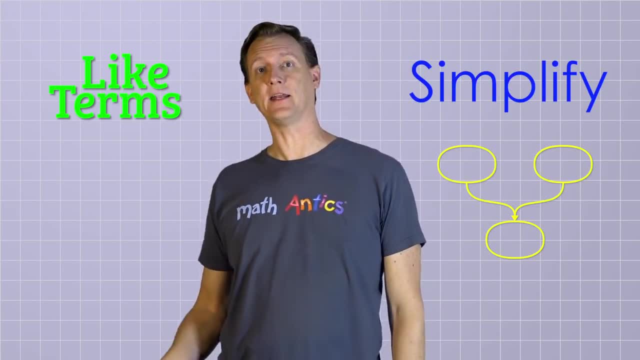 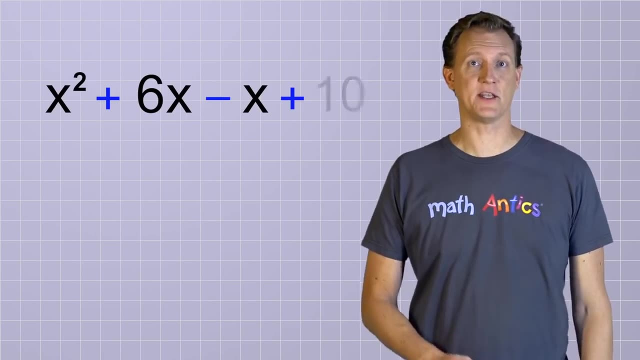 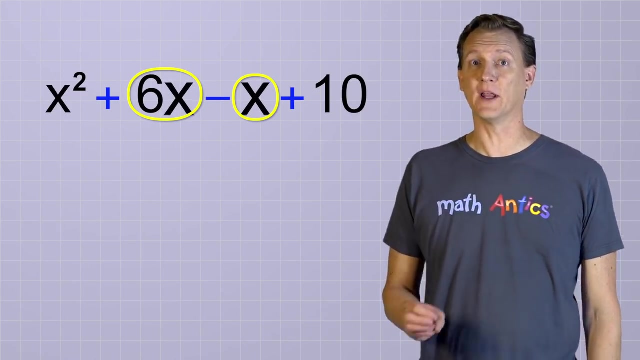 complicated polynomials that we can simplify by combining any like terms that we find. Here's our first example: x squared plus 6x minus x plus 10.. Do you see any terms that have the same variable part? Yup, these two terms in the middle both have the variable x, so we can combine them. 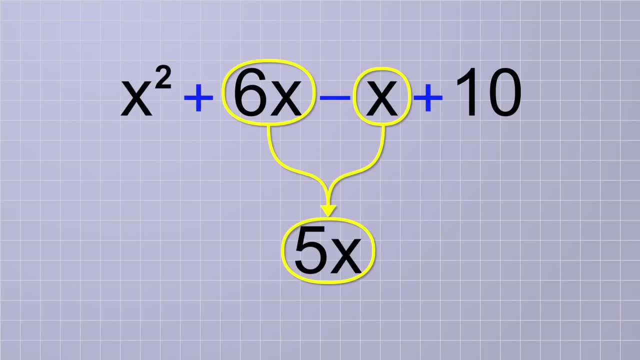 6x minus x would just get…. 6x would just give us 5x, since 6 minus 1 is 5.. Remember: if you don't see a number part in a term, then it's just 1.. So this polynomial started with 4 terms, but simplified to 3 terms. 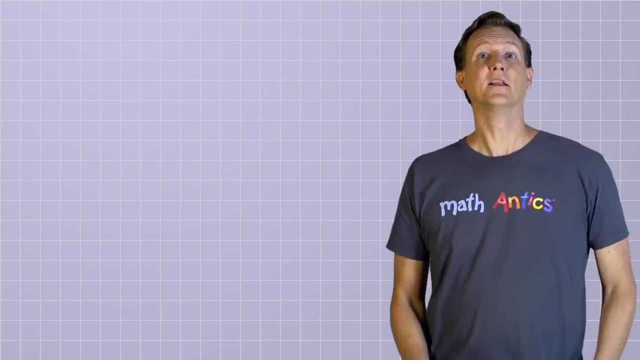 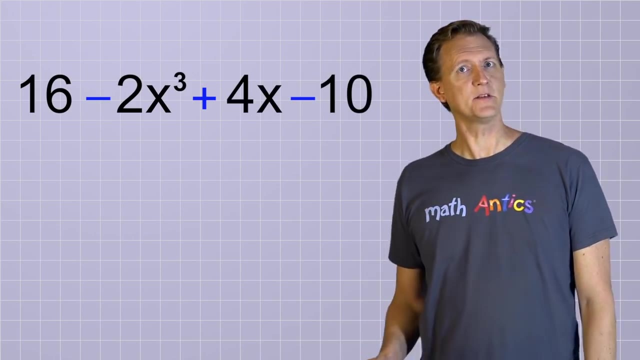 x squared plus 5x plus 10.. Let's try this one: 16 minus 2x, cubed plus 4x minus 10.. In this polynomial we have a third degree term, a first degree term and two constant terms. 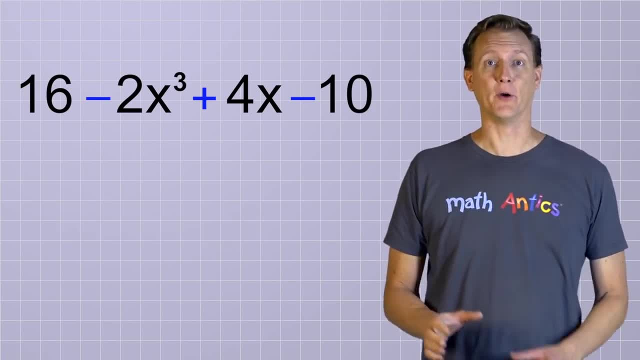 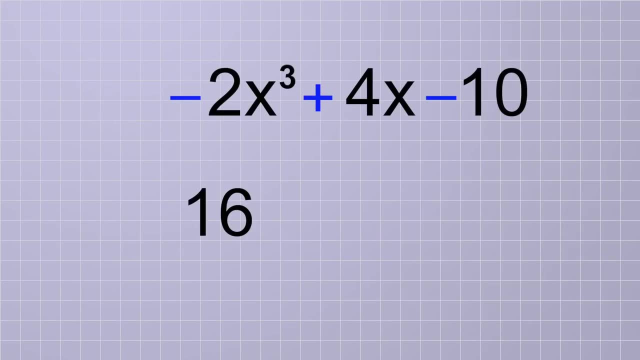 Are those constant terms like terms? Absolutely, They're both just numbers and don't really have a variable part. so we can combine them easily. This term is positive 16 and this term is negative 10. So if you add them together you end up with positive 6.. 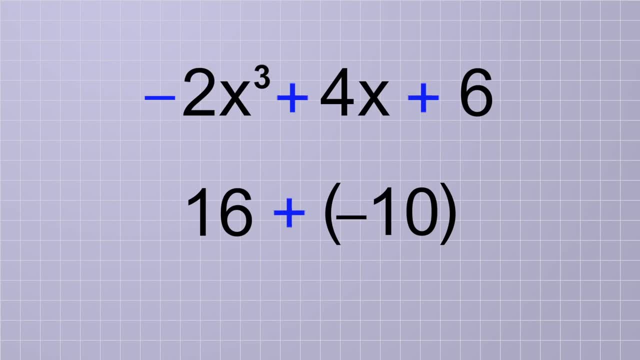 Remember, it's best to think of all terms in a polynomial as being added, but they can have coefficients that are either positive or negative. That's why this negative sign stays here, with the 2x cubed term… because it's a negative term. 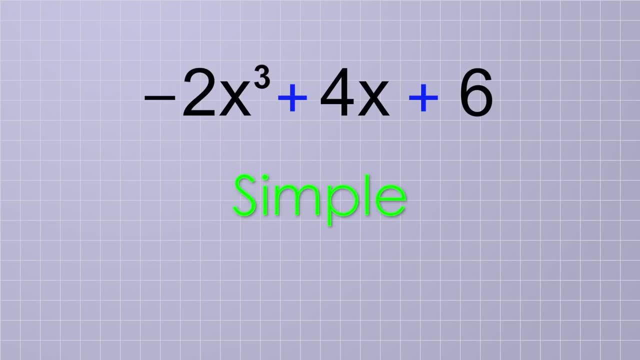 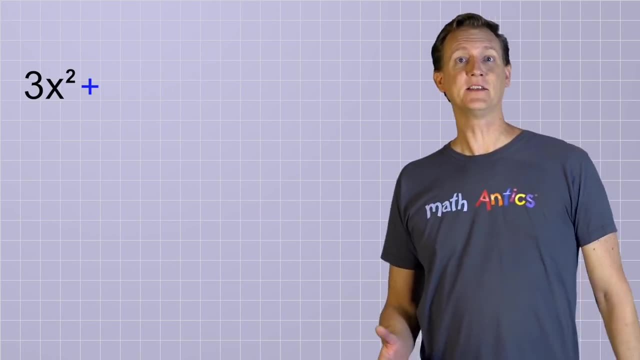 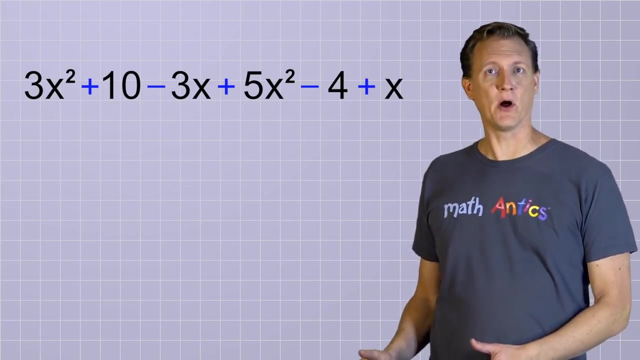 So this polynomial is now as simple as it can be, since there's no other like terms Ready for an even more complicated polynomial: 3x squared plus 10 minus 3x plus 5x squared minus 4 plus x, This polynomial has 6 terms. 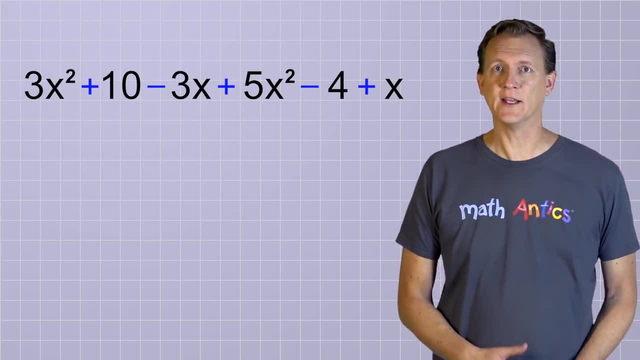 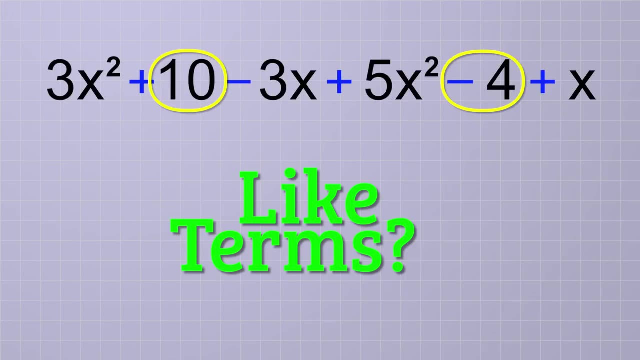 And when you get a long polynomial like this, the first thing to do is look to see if any of the terms are like terms so you can combine them Well…. You may notice that there's two constant terms in this polynomial: positive 10 and. 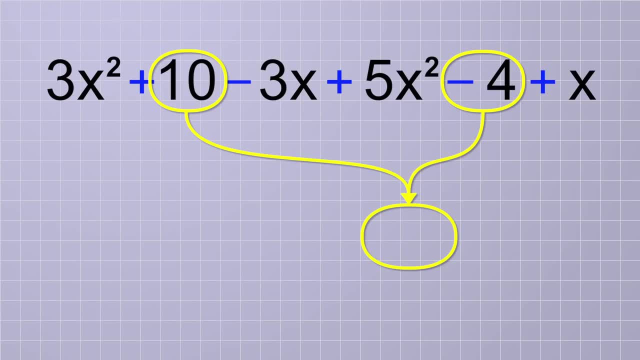 negative, 4.. So let's start by combining them into a single constant term: positive 6,, since 10 minus 4 equals 6.. Next, we see that there are also two first degree terms, negative 3x and positive x. 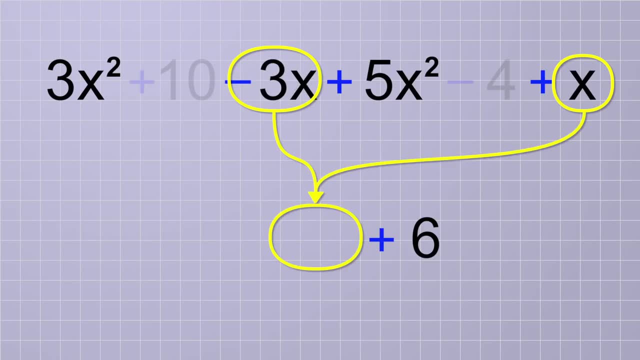 Those are like terms, so we can combine them. Negative 3x plus 1x gives us negative 2x. Last, we see that there's also two different terms that have the variable part x squared, So we can combine them too.